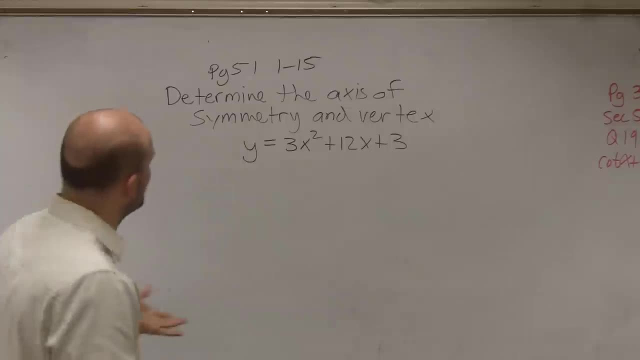 Okay. So, ladies and gentlemen, what this problem asks us is, it says: determine the axis, symmetry and the vertex. So, please, this is what I'd like you guys to do. Until you really get good at doing these type of problems, please, let's write down exactly. 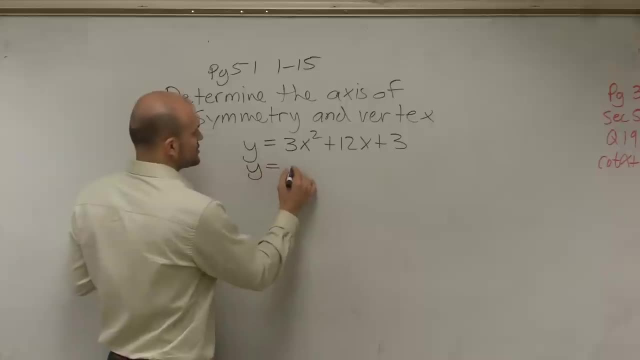 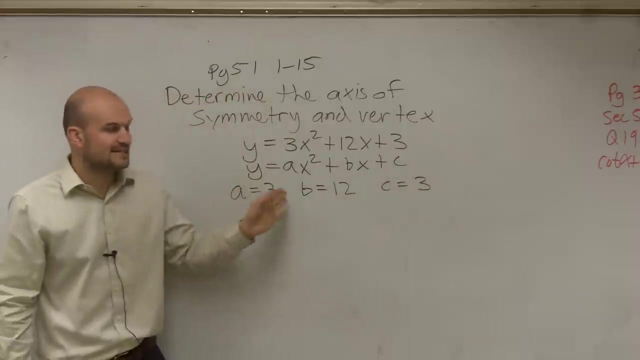 what our a, b and c are. Remember. every quadratic equation can be written in the form of ax squared plus bx plus c. Therefore, in this problem, we can say: a equals 3,, b equals 12, and c equals 3.. Right, As each one of these values are real numbers and either 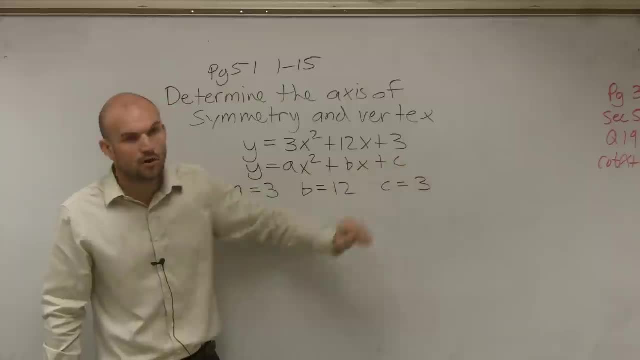 the coefficients of our quadratic or linear term are our constant. Does everybody see how I got those values? Okay, So now there's two formulas that we first need to work with. The first formula is what we call the axis of symmetry. So the axis of symmetry is simply: 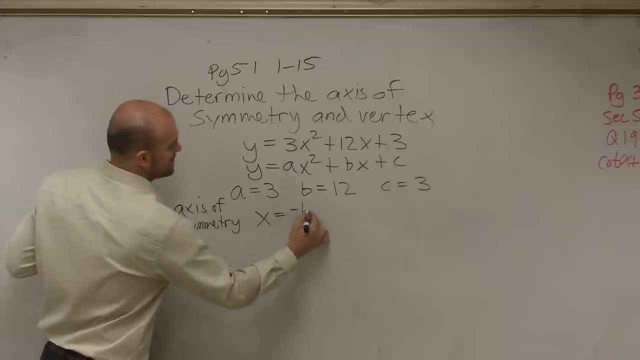 just say it's x equals, because it's a vertical line- equals epsilon. So the axis of symmetry is the opposite of b divided by 2 times a. So all I'd like you guys to do to find the axis of symmetry is just take the opposite of b, which is negative. 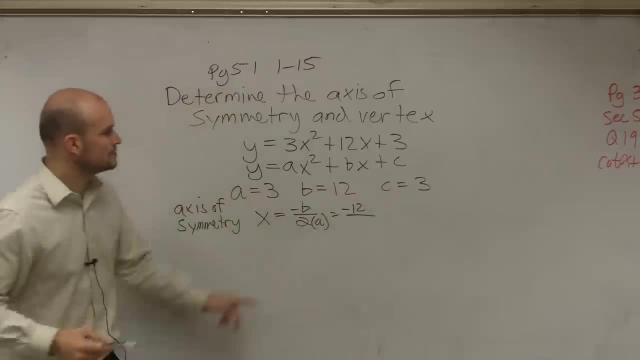 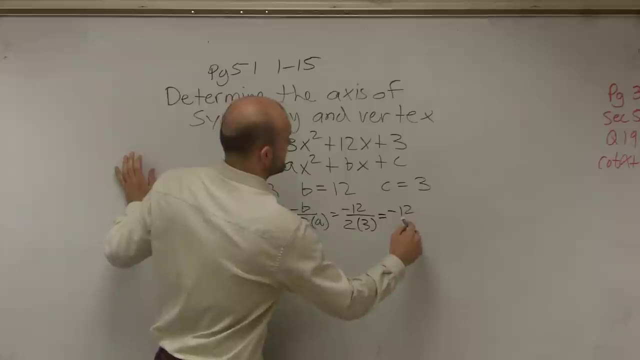 12, divided by 2 times a. Well, 2 times a is 2 times 3.. Therefore, it's negative 12 divided by 6, which equals negative 2.. And about half the class got to this point. Alright. 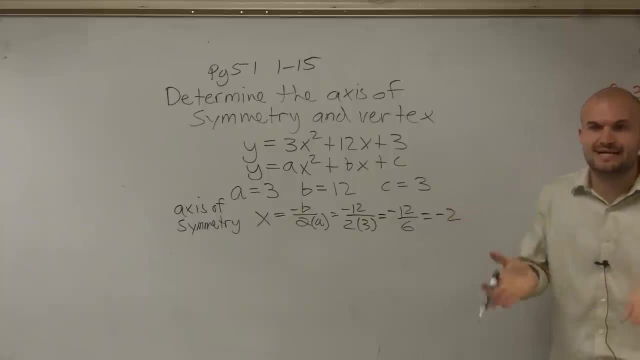 And that's where you want to fit in. So what that is is that's the axis of symmetry, That is, the vertical line that your parabola can be reflected about, is symmetrical about, But that's not the whole part of the vertex. 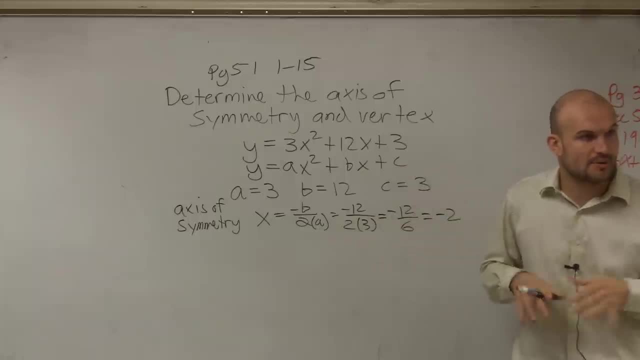 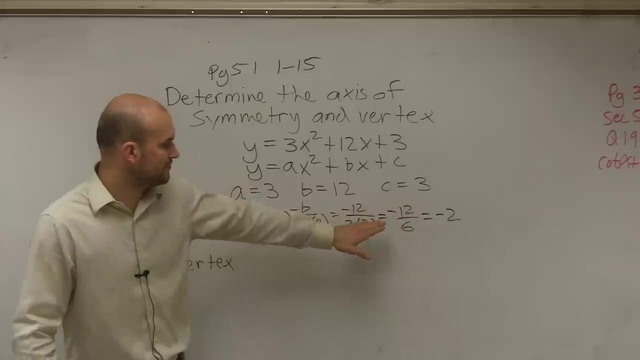 The axis of symmetry goes through your vertex. Remember, the vertex is either maximum or minimum variable parabola. So to determine the vertex, what we need to do is this: Yeah, kind of This is your. so, once you know the vertex, 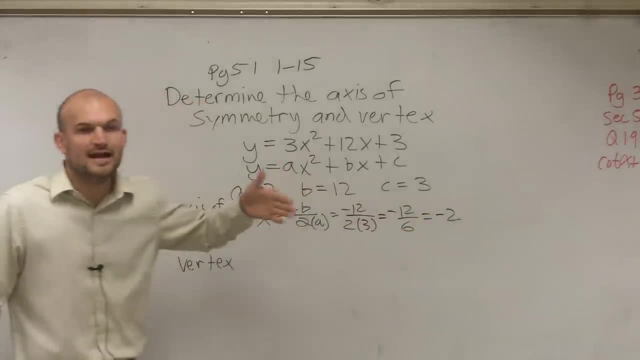 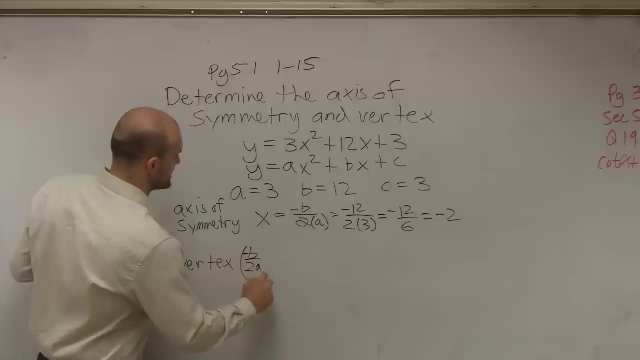 or, I'm sorry, the vertex. this is your x value of your vertex. We need now to find the y value of vertex. So the vertex has the formula of b divided by opposite of b divided by 2 times a, which is the x value. 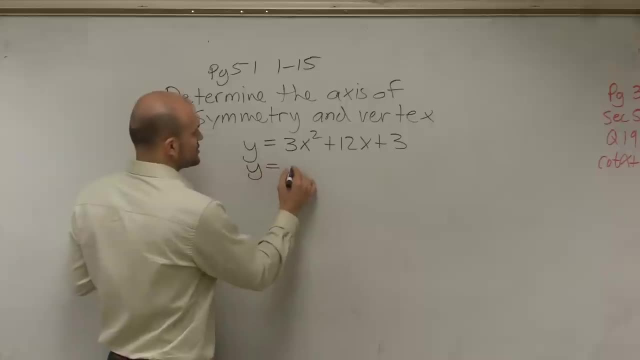 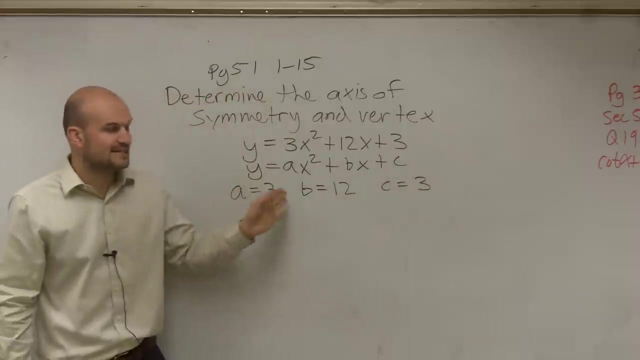 what our a, b and c are. Remember. every quadratic equation can be written in the form of ax squared plus bx plus c. Therefore, in this problem, we can say: a equals 3,, b equals 12, and c equals 3.. Right, As each one of these values are real numbers and either 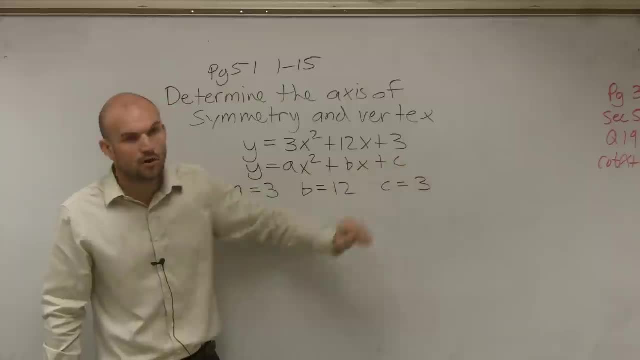 the coefficients of our quadratic or linear term are our constant. Does everybody see how I got those values? Okay, So now there's two formulas that we first need to work with. The first formula is what we call the axis of symmetry. So the axis of symmetry is simply: 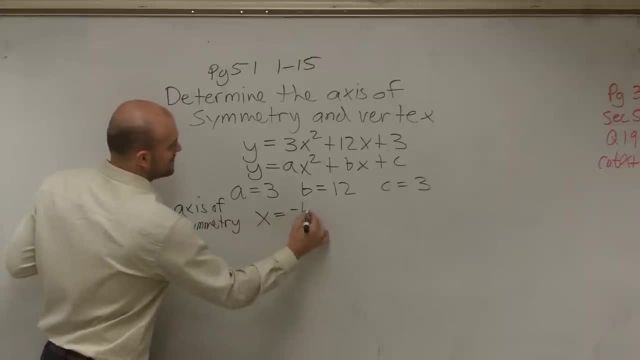 just say it's x, equals because it's a vertical line- equals epsilon. So we're going to take the opposite of b divided by 2 times a. So all I'd like you guys to do to find the axis of symmetry is just take the opposite of b, which would be: 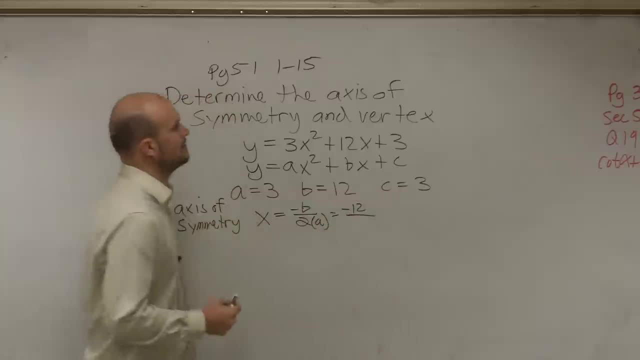 negative 12, divided by 2 times a. Well, 2 times a is 2 times 3.. Therefore, it's negative 12 divided by 6, which equals negative 2.. And about half the class got to this point. 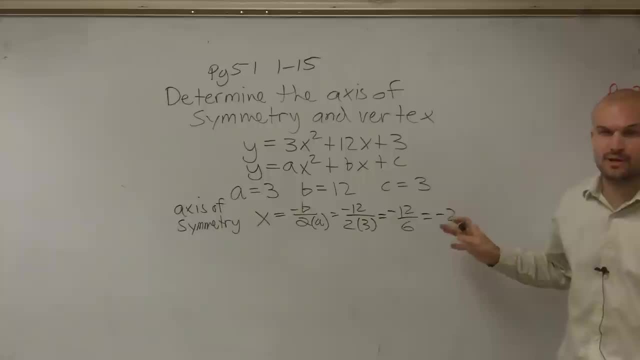 All right, And that's where you want to fit in. So what that is is: that's the axis of symmetry, That is, the vertical line that your parabola can be reflected about, is symmetrical about, But that's not the whole part of the vertex. 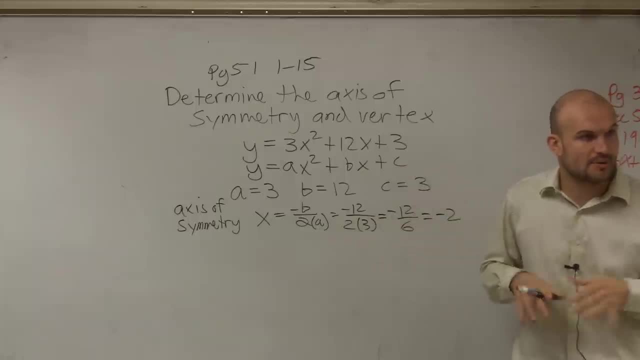 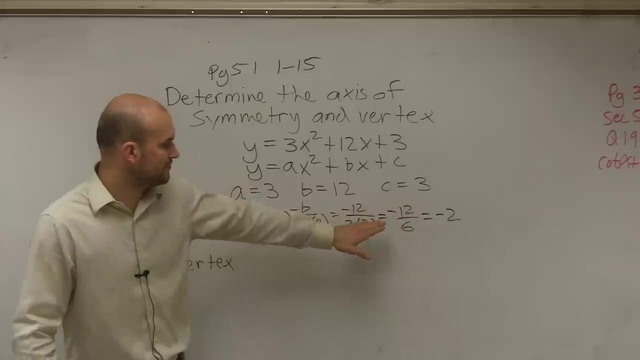 The axis of symmetry goes through your vertex. Remember, the vertex is either maximum or minimum variable parabola. So to determine the vertex, what we need to do is this: Yeah, kind of This is your. so, once you know the vertex, 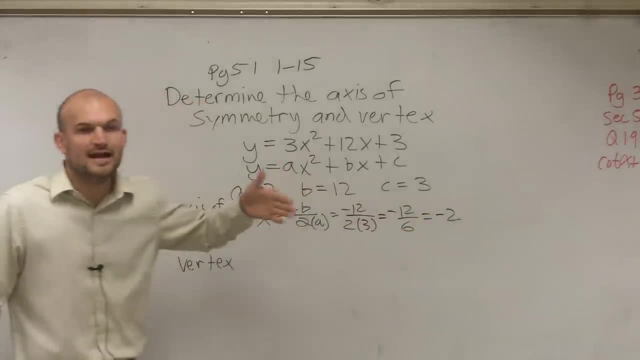 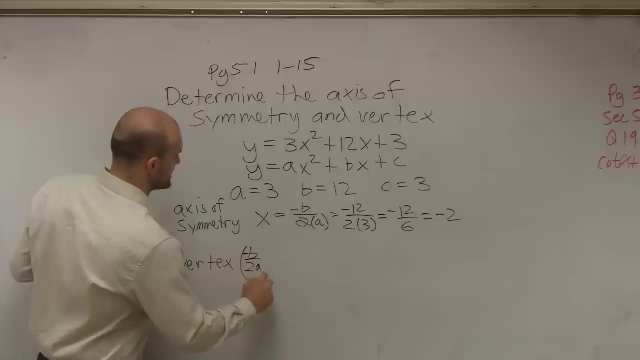 or, I'm sorry, the vertex. this is your x value of your vertex. We need now to find the y value of vertex. So the vertex has the formula of b divided by opposite of b divided by 2 times a, which is the x value. 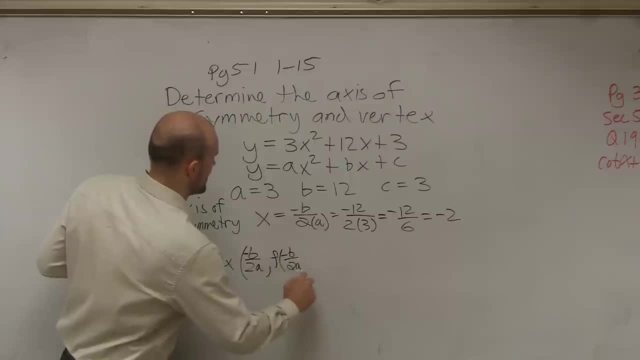 And then it is f of opposite of b divided by 2a, And you might say, well, that kind of looks a little crazy. What exactly am I doing? All? we're not dealing with a function, We're actually just dealing with an equation. 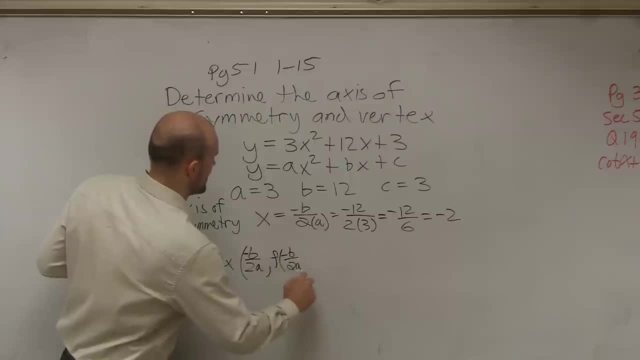 And then it is f of opposite of b divided by 2a, And you might say, well, that kind of looks a little crazy. What exactly am I doing? All? we're not dealing with a function, We're actually just dealing with an equation. 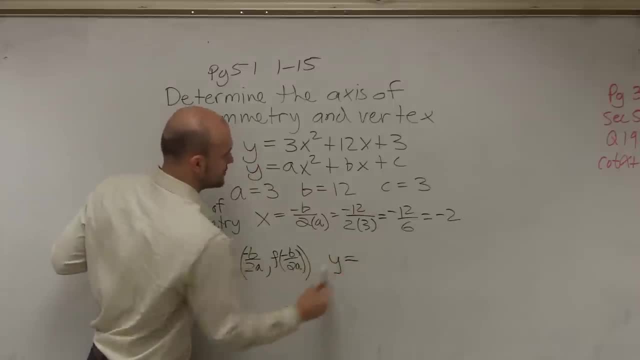 But what you're going to do is simply just take your value for x and plug it into your equation, So I'll have 3 times negative 2 squared plus 12 times negative 2 plus 3.. And here's where negative 2 is your value of x. 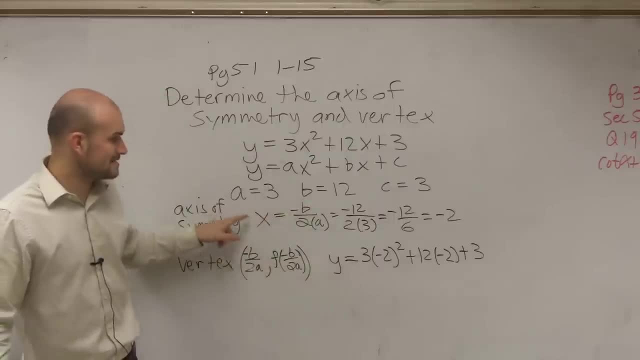 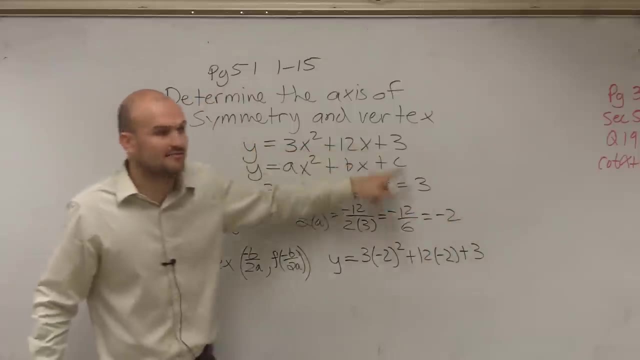 Right. So remember, we found the axis of symmetry, which x is the value of x. x equals negative 2.. So then what we do is we plug negative 2 in for x to find our y value. Yes, Where is negative 2 squared? 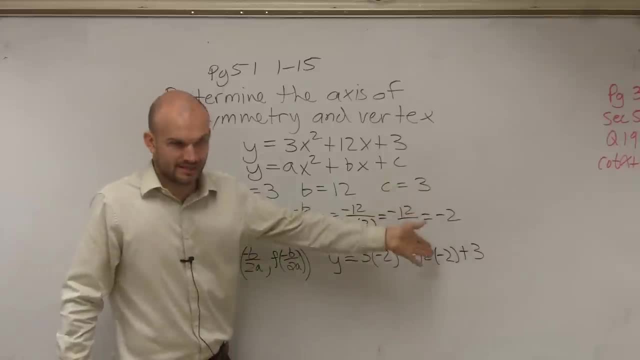 Oh, that's y equals. oh, you're plugging it back in. I'm plugging it into the equation for x. Now, here's where a lot of students made the mistakes and you guys are going to want to remember this. 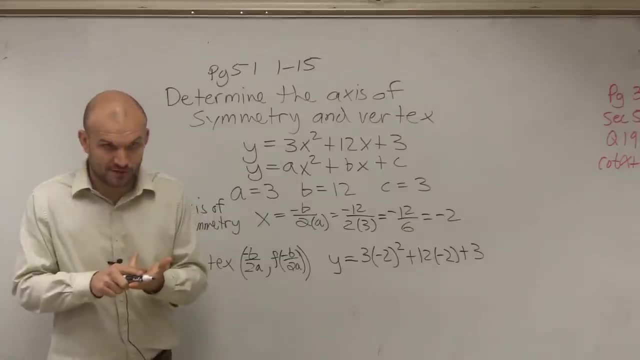 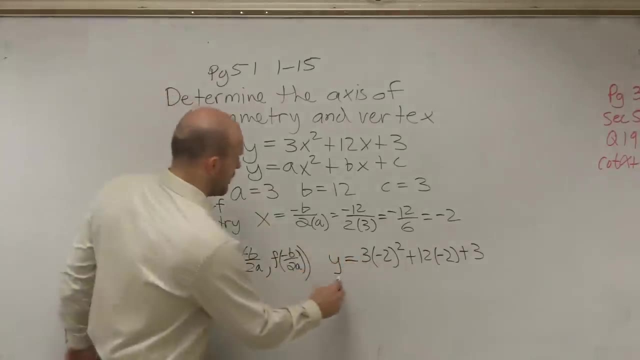 Order of operations. Parentheses or grouping terms first, Then exponents and powers. Ladies and gentlemen, you have to square this first, So it's going to be y equals 3 times 4. Plus you can multiply those. 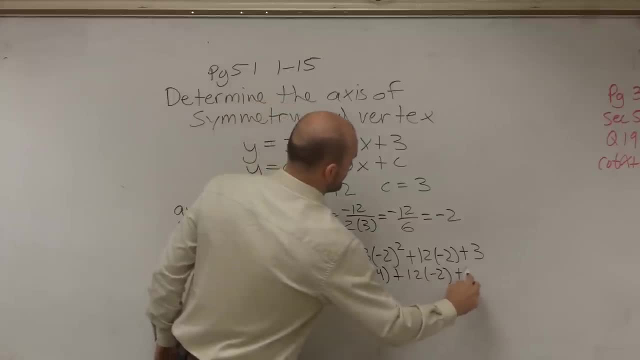 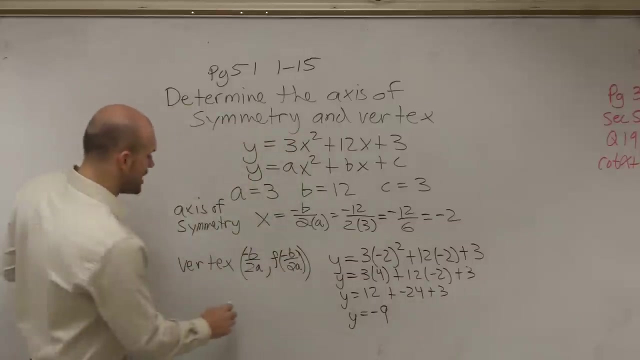 which would be: or 12 times negative, 2 plus 3. Now you do multiplication and division: y equals 12 plus negative, 24 plus 3. Therefore y equals negative 9.. Now you can say your vertex has an x coordinate of negative 2. 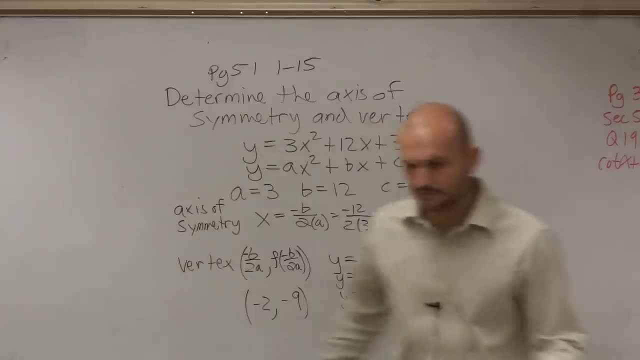 and a y coordinate of negative 9. how do you figure out what the end? you just go: 12 plus negative 24 is negative 12 and then negative 12 plus 3 is going to be named. I'm you always work from left to right? yes, this is just exactly what we did. we found what the X. 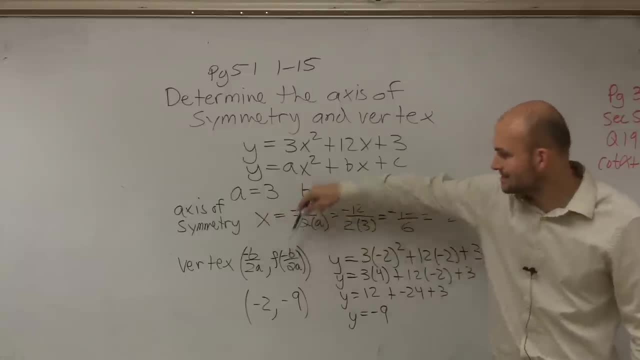 value is. and then what we did is we plug the X value into our equation, and this in the formula. this is for plugging it back into the function, which is the same thing. all it means is find your value for X and then plug it into the equation. 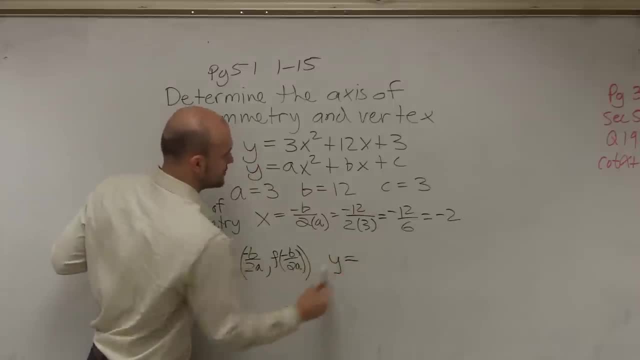 But what you're going to do is simply just take your value for x and plug it into your equation, So I'll have 3 times negative 2 squared plus 12 times negative 2 plus 3.. And here's where negative 2 is your value of x. 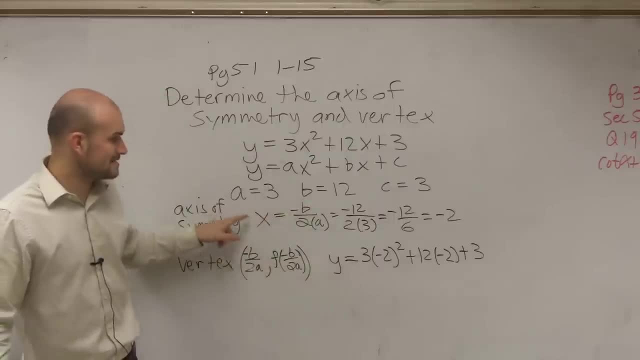 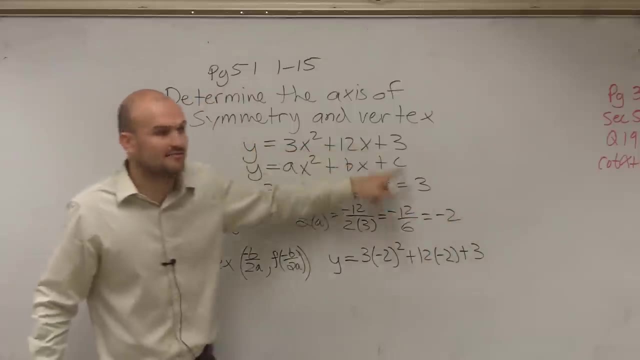 Right. So remember, we found the axis of symmetry, which x is the value of x. x equals negative 2.. So then what we do is we plug negative 2 in for x to find our y value. Yes, Where is negative 2 squared? 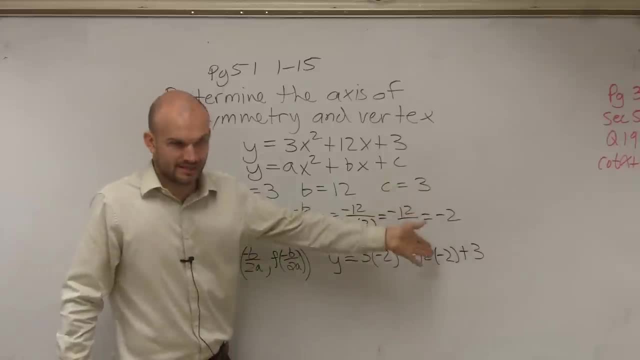 Oh, that's y equals. oh, you're plugging it back in. I'm plugging it into the equation for x. Now, here's where a lot of students made the mistakes and you guys are going to want to remember this. 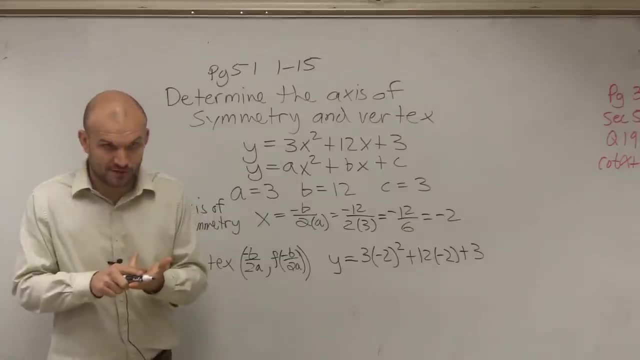 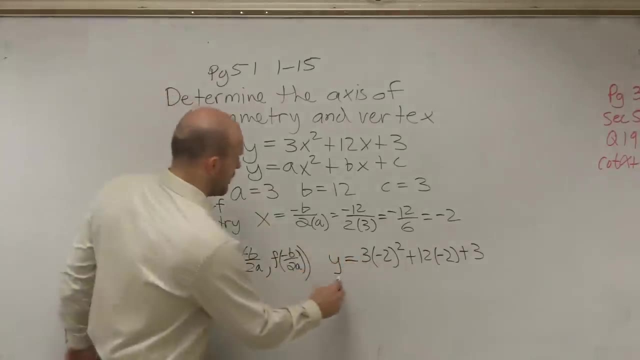 Order of operations. Parentheses or grouping terms first, Then exponents and powers. Ladies and gentlemen, you have to square this first, So it's going to be y equals 3 times 4. Plus you can multiply those. 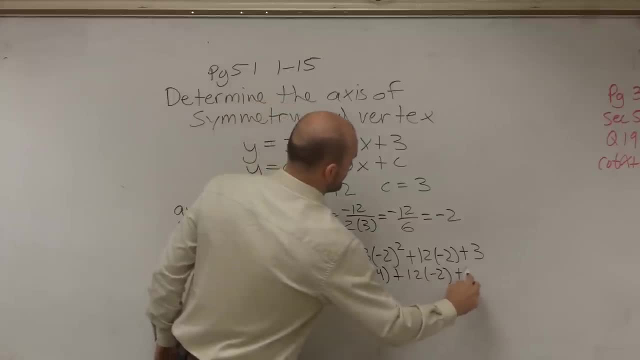 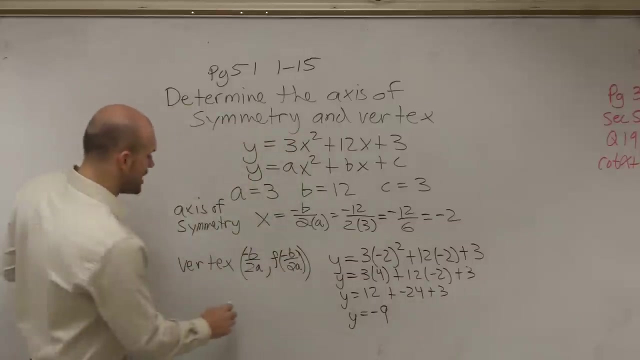 which would be: or 12 times negative, 2 plus 3. Now you do multiplication and division: y equals 12 plus negative, 24 plus 3. Therefore y equals negative 9.. Now you can say your vertex has an x coordinate of negative 2. 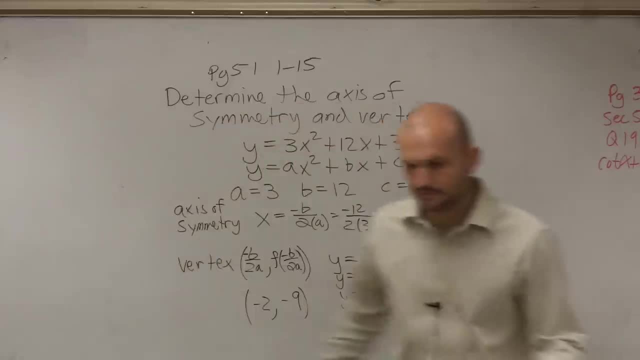 and a y coordinate of negative 5.. Therefore you have y equals 8.. of negative 9, how do you figure out what the answer? you just go: 12 plus negative 24 is negative 12 and then negative 12 plus 3 is going to be negative you. 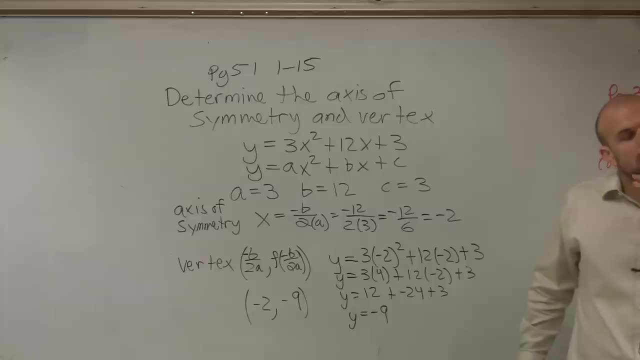 always work from left to right. yes, this is just exactly what we did. we found what the x value is, and then what we did is we plug the x value into our equation, and this in the formula. this is for plugging it back into the function, which is the same thing. all it means is find your value for X and then plug it. 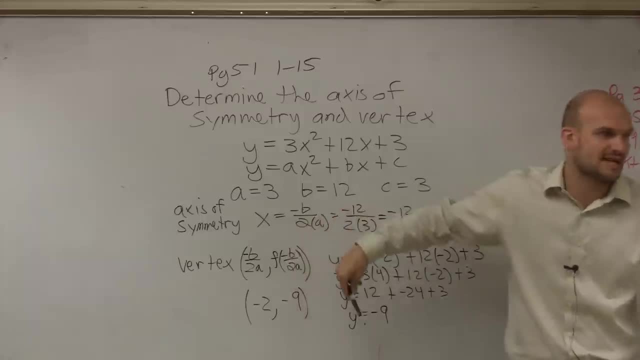 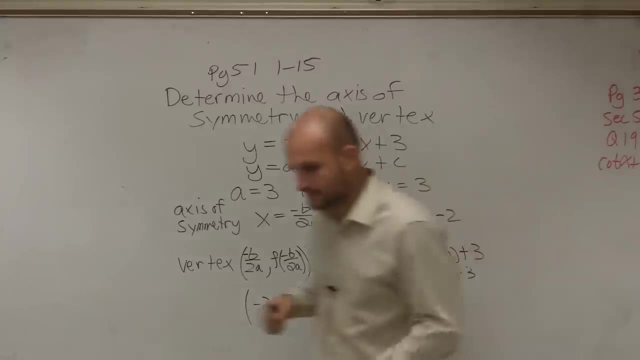 into the equation or function to find the Y. so that's just exactly what we did. it's just kind of the formula that you can use. anybody have any questions? no, okay, I know you did it wrong.